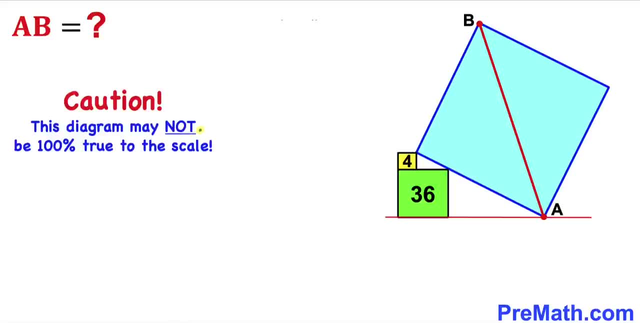 Please don't forget to give a thumbs up and subscribe. Please keep in mind that this figure may not be 100% true to the scale. Let's go ahead and get started, And here is our action plan. We are going to calculate the side length of this blue square before we calculate the diagonal A, B, And here's our very first step. Let's focus on this yellow square, whose area is 4.. 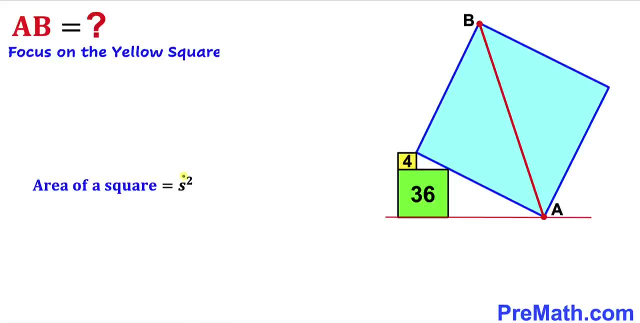 And now let's recall the area of a square, formula: Area equal to S square, where S represents the side length of the square. So, therefore, the side length of this yellow square is going to be 2, since 2 square is going to give us 4.. As you can see over here, the side length of this yellow square is 2.. And now let's focus on this green square, whose area is 36.. And once again we are going to apply this: 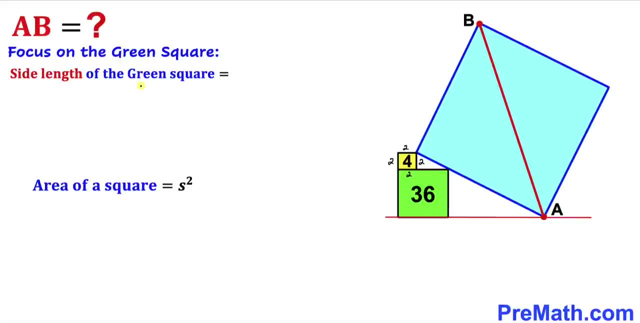 formula: area of square formula. So, therefore, the side length of this green square turns out to be 6, since 6 square is going to give us 36.. As you can see over here, the side length of this green square is 6 across the board. And here's our next step. We have labeled these points as 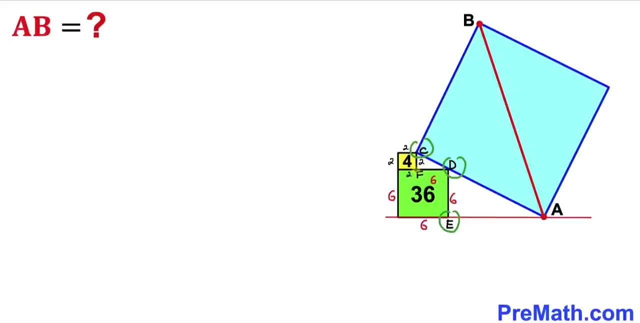 C, D, E and F. And now our task is to calculate these individual side lengths: C, D, and then this D, A, And now we know that this whole side length is 6 and this tiny side length is 2.. Therefore, 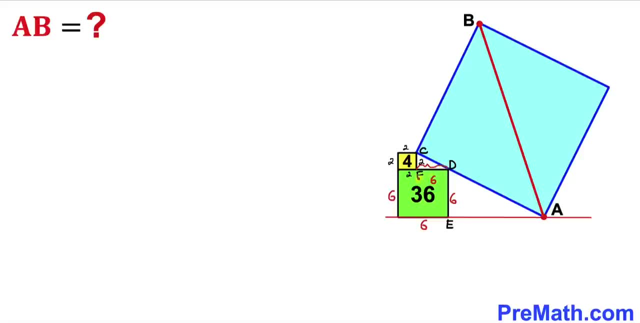 this F D length is going to be 6 minus 2 is going to give us 4.. And furthermore, let's assume that this side length, E, A is x units. And now our task is to calculate this value of x. And here's our next step. Let's focus on these two right triangles. 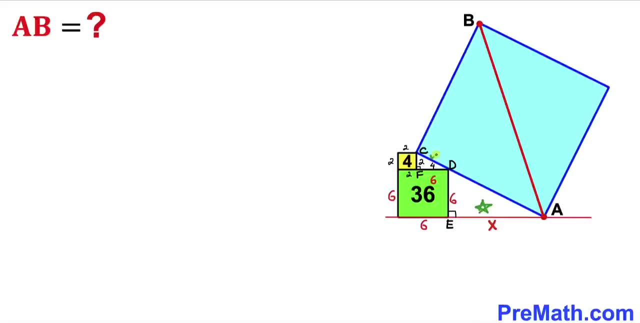 A, E, D, and this another right triangle, D, F, C, and these two angles are 90 degrees. So therefore we conclude that these are two right triangles- AED and this other right triangle, DFC- are similar triangles according to angle angle similarity theorem, because these angles are 90 degrees each. 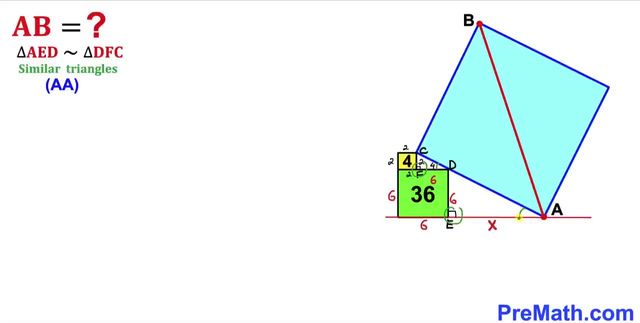 and these are our corresponding angles. so therefore, we are going to have a proportions. so the ratio of x and 6- let me go ahead write down x divided by 6- is going to be equal to the ratio of 4 and 2. let me go ahead, write down 4 divided by 2. let's go ahead and multiply both. 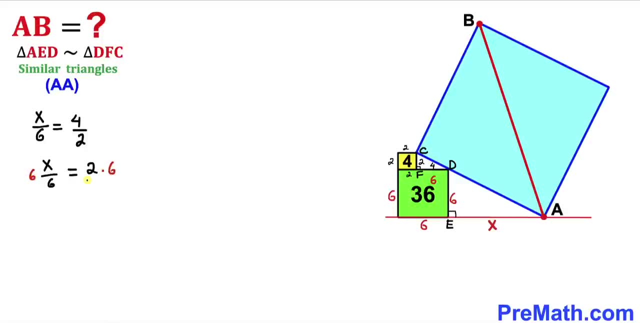 sides by 6 to isolate x. this 6 and 6 is gone, so therefore our x value turns out to be 4- 12, so therefore I can replace this x by 12 over here. in other words, our EA length turns out to be 12. and here's our next step. let's focus on this right triangle, AED, whose side lengths are 12. 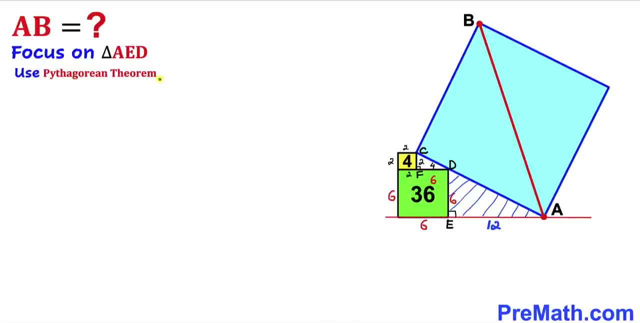 and 6, and now we are going to use the Pythagorean theorem to find the value of this side, length DA. and here's our Pythagorean theorem. let me go ahead and call this longest leg as side C, this side A and this side B. go ahead and. 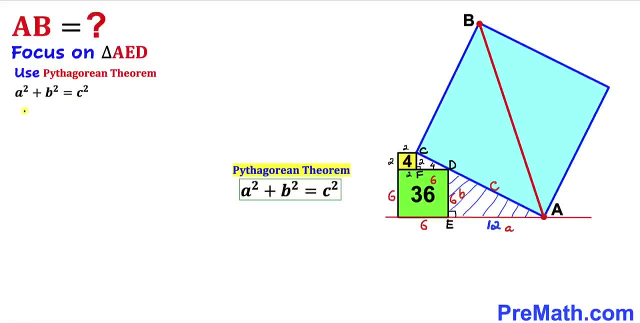 fill in the blanks in this formula. so A square is going to be 12 square plus B. in our case is 6 square equal to C square, so therefore C square value turns out to be 180. let's go ahead and undo this square and we are going to have 12 square plus B, and we are going to have 12 square. 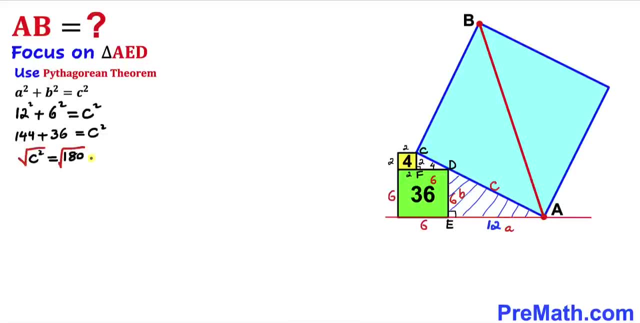 by taking the square root on both sides, and here we can see this square and square root is gone. so C equal to. and now let's focus on this right hand side, and here I have copied down square root of 180, and if we simplify this one, it turns out to be 6 times square root of 5. so therefore our C. 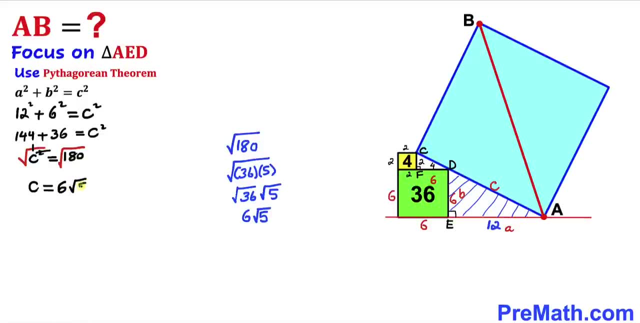 value turns out to be 6 times square root of 5.. So, therefore, our DA length turns out to be 6 times square root of 5.. And here's our next step. Let's focus on this. another right triangle, DFC, And we are going to use the Pythagorean theorem once again to find the value of this. 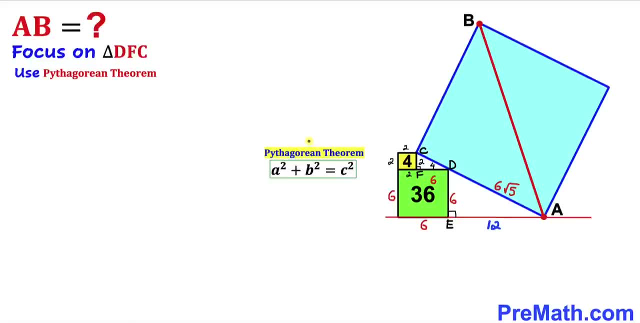 side CD. And here's our Pythagorean theorem. once again, A square plus B square equal to C square. Let me go ahead and call this longest leg as our side C. I'm going to call this side A and this B. Let's go ahead and fill in the blanks. So A square is going to be 4 square plus B is 2 square equal. 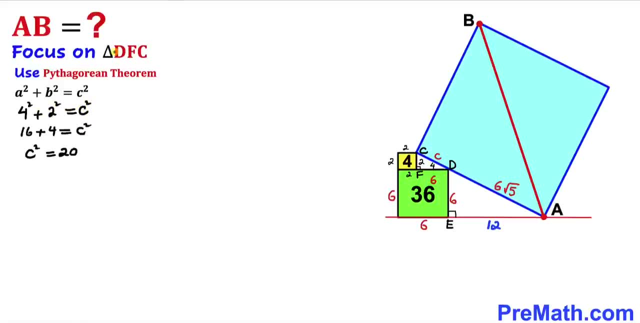 to C square. Let's go ahead and undo this square by taking square root on both sides. So, therefore, our C value is going to be equal to: And now let's focus on this right hand side. I have just copied down this square, So let's go ahead and undo this square by taking square root on both sides. 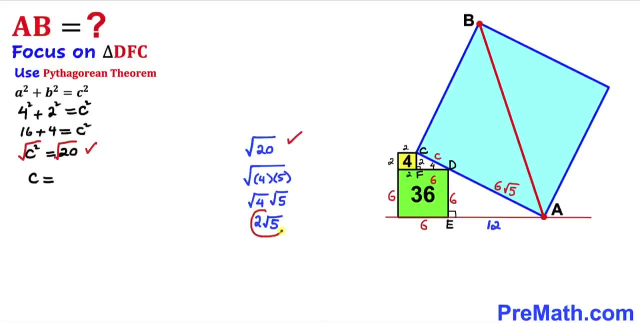 Square root of 20.. And if we simplify, that is going to be equal to 2 times square root of 5.. So, therefore, C is going to be equal to 2 times square root of 5.. So, therefore, our this side length, CD, is going to be 2 times square root of 5.. And here's our next step. Let's focus on this. 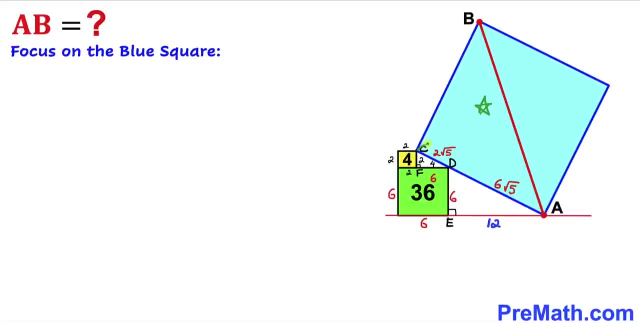 blue square now And we are going to calculate this side length of this blue square. So, therefore, the side length of this blue square is going to be a 2 times square root of 5, plus this length, 6 times square root of 5.. We're going to add them up, So, therefore, the side length of this blue square 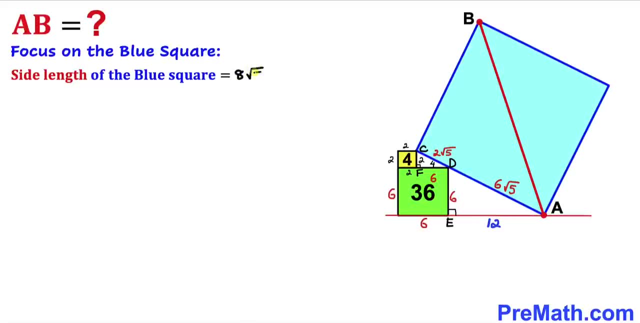 turns out to be 8 times square root of 5.. And since we are dealing with the square, So all these side lengths of this blue square are going to be 8 times square root of 5 across the board. And in this next step, let's focus on 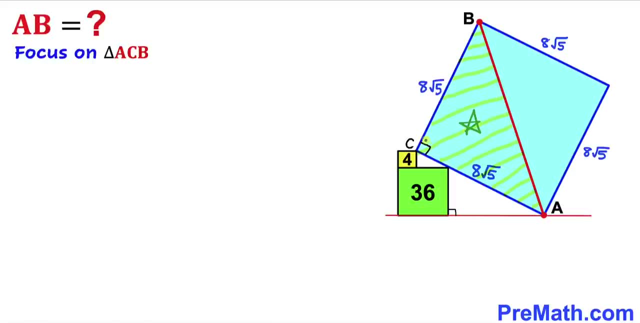 right triangle ACB, and we know that this angle is 90 degrees, since we are dealing with the square and we are going to use the Pythagorean theorem. and here's our Pythagorean theorem: a square plus B square, equal to C square. let me go ahead.